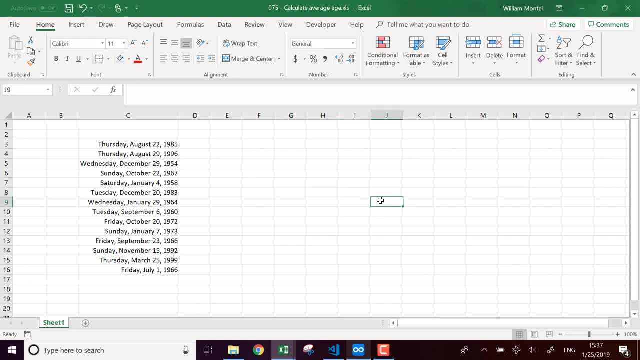 Hello Excel Champions. it's William, aka DrExcel. Today I'm going to show you how to calculate the average age for a list of people. So here I have a list of date of birth. I want to calculate the average age of those people. 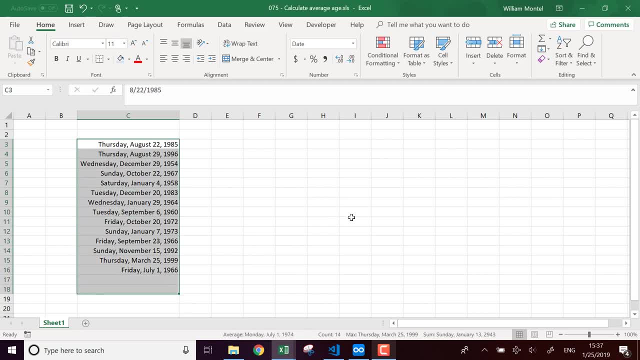 So I'm going to show you how to do this with formulas and I will give you the file which is going to be right below the video. You can download it. There's a link So you can download it and follow with me with all the formulas. 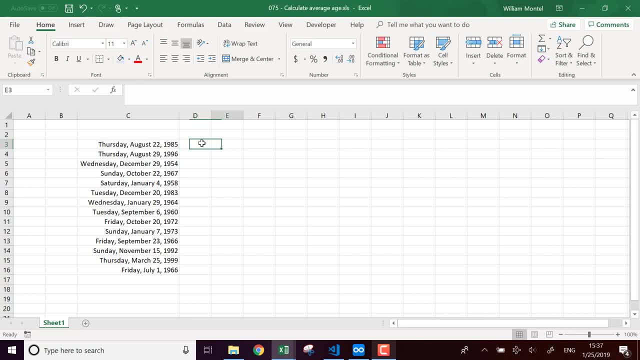 So what I'm going to do for each person, I'm going to compute the person's age, So I'm going to use the date of birth, which is actually today minus the date of birth. Why do I do this? Because actually dates, So today returns the date of today. 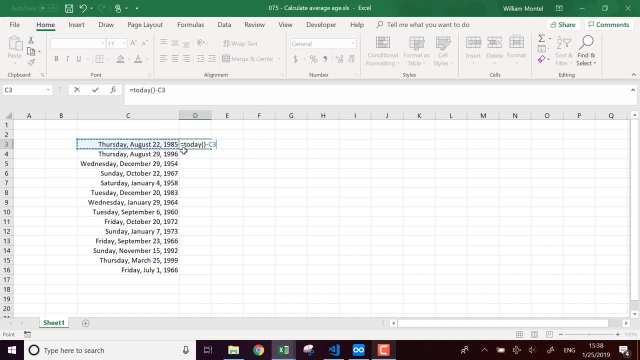 And the date of birth. actually dates in Excel are just numbers. They are the number of dates, The number of days that have passed since January 1st 1900.. So it's just a number of days. I can make operations on them. 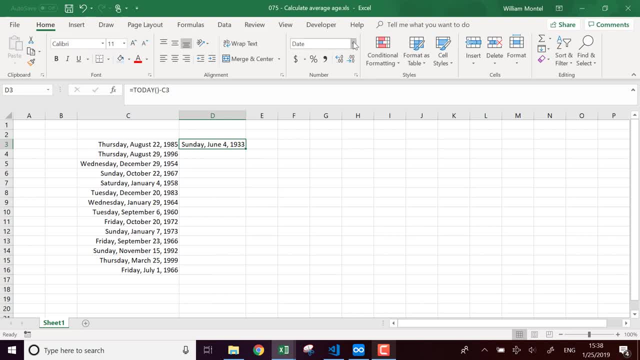 And I'm going to subtract them. So here this doesn't mean anything because it's a difference between two dates, between today and that date in a number of days. So here that's number of days. I can make the average of that. 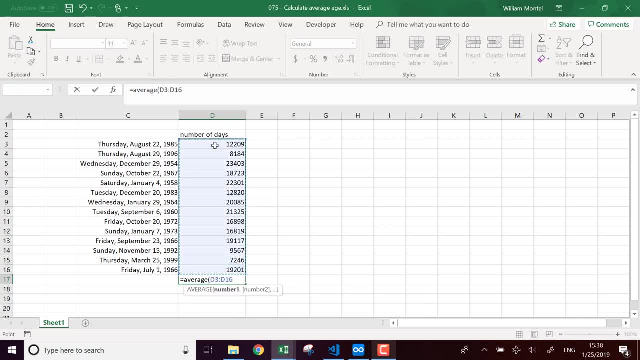 So I'm going to make average this, And this is the average age of these people, but in terms of days, So this is actually a date. So now, if I want to express this, this average age, not in days but in years, for example, I'm going to use the function date diff. 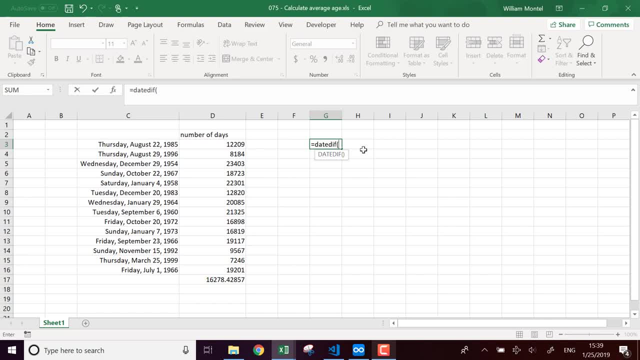 Date diff, which is like a hidden function. It's not very well explained in Excel And I'm going to compute the difference. The function date diff. it tells the difference between two dates in terms of year, month or days. And here what I'm going to do, I'm going to make the difference between 0 and this number of days.